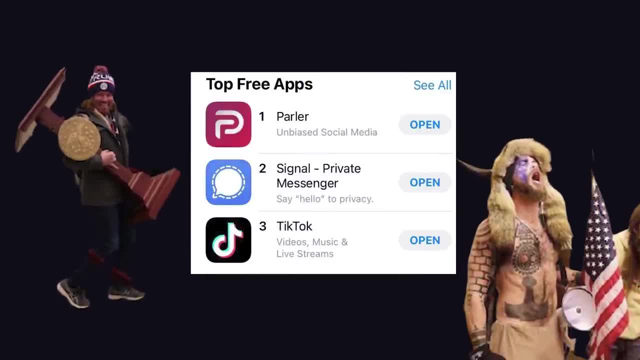 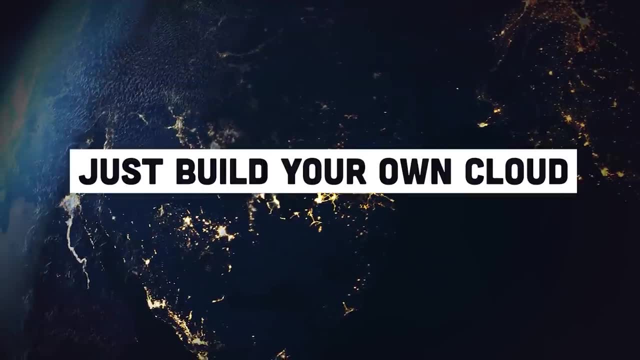 This week in tech, Amazon took the fastest growing social media app of all time and migrated it to its new serverless platform, putting it in the highly undesirable position of requiring a reverse cloud migration. Most companies migrate from on-prem to the cloud, but this unfortunate app needs to do the exact opposite, because nobody in town wants to touch it. Whether you agree with the politics of that or not, one thing is undeniable: Tech monopolies have a lot of power over your business, So don't walk around here thinking you have free will. because you don't. I can crush you. 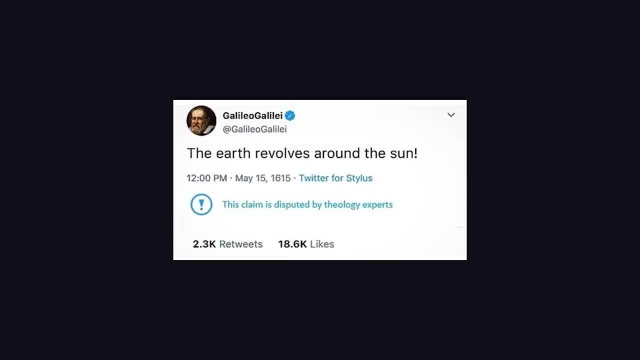 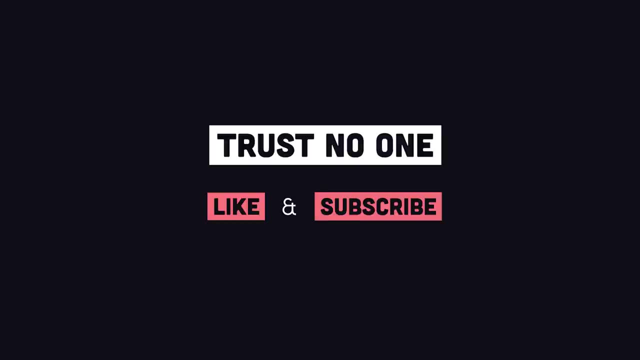 anytime I want And a lot of influence over the content we consume as end users. That being said, if you're some kind of f***ing weirdo who doesn't trust the cloud, this video is for you. We'll take a Raspberry Pi and turn it into a physical server that can host a web application on the internet. 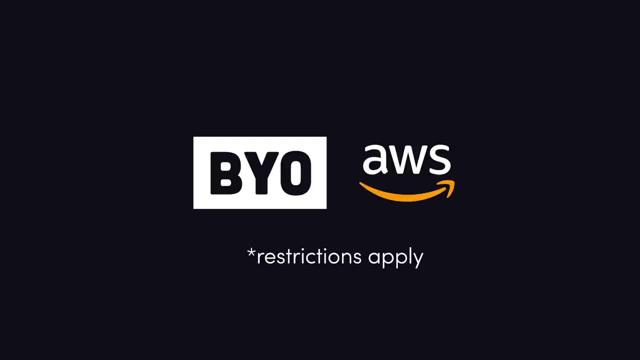 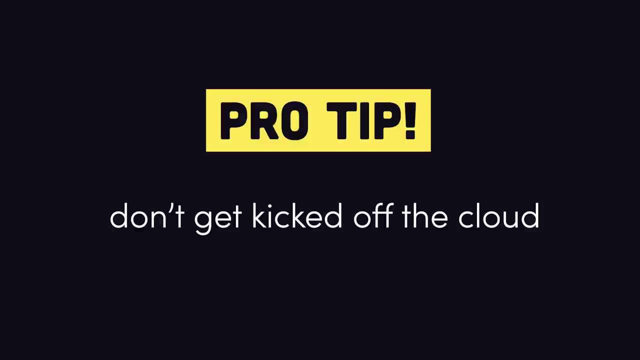 Or in other words, you'll build your own mini Amazon web services from scratch. Along the way, you'll learn some cool things about Linux, networking, Nginx, Nodejs and why if you have a large-scale app and get kicked off of AWS, you're pretty much screwed To follow along. 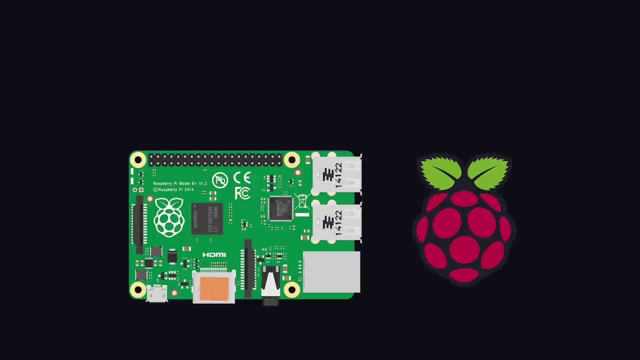 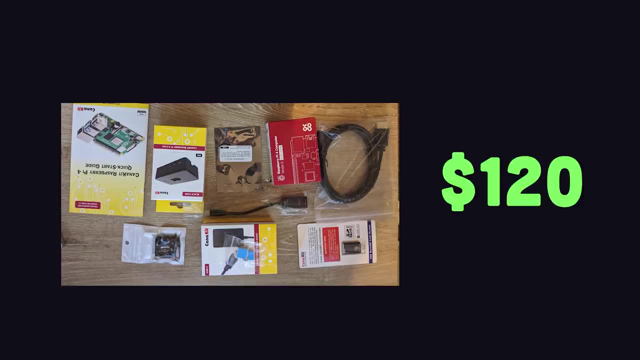 the first thing you'll need is a Raspberry Pi. I'm using the Model 4,, which has a quad-core processor and 8 gigabytes of RAM. Unironically, I bought it as a kit from Amazon for about 120 bucks. It comes with a power supply, all the cords you need, as well as a memory card with. 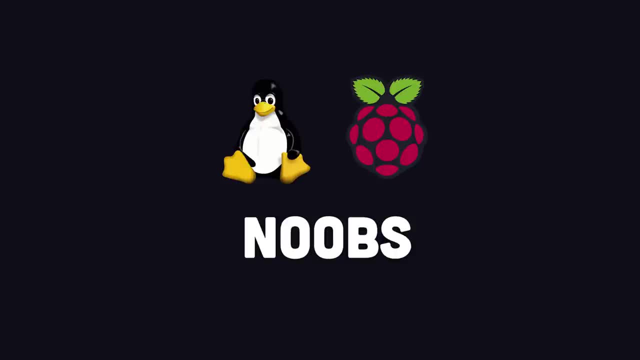 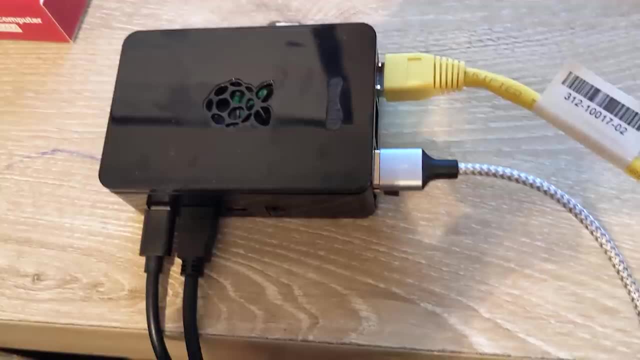 Linux pre-installed. The Linux flavor is designed specifically for Raspberry Pi. It's called Noobs and feels pretty similar to Ubuntu. Now, I'm not going to go through the physical hardware setup here, which is really just a matter of plugging in different sized cords to different sized holes. 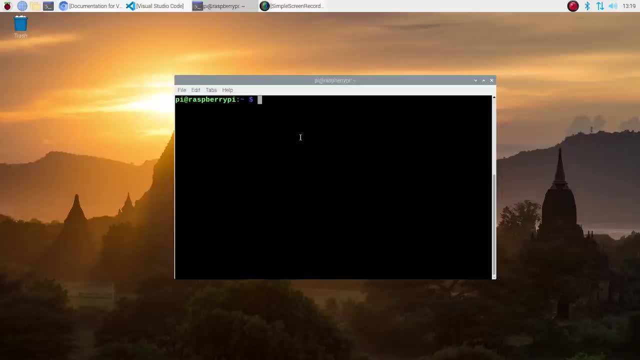 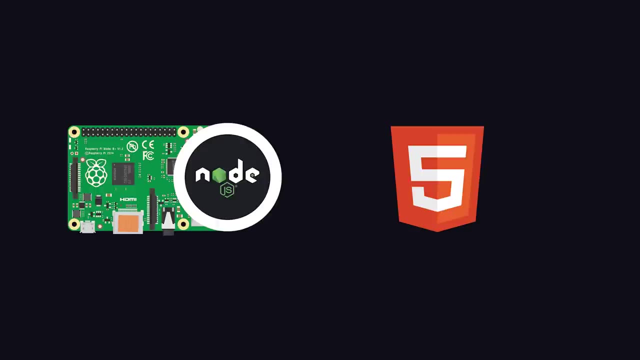 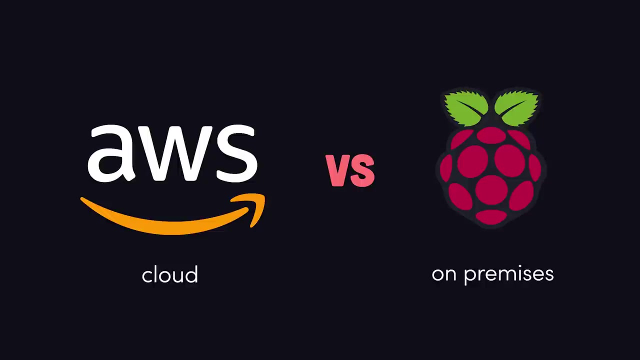 Now our goal here is to create a Nodejs web application that can serve HTML from the Raspberry Pi to the rest of the internet throughout the world. But before we do that, let's talk about some of the challenges and how it compares to hosting a website on the cloud. The first issue: 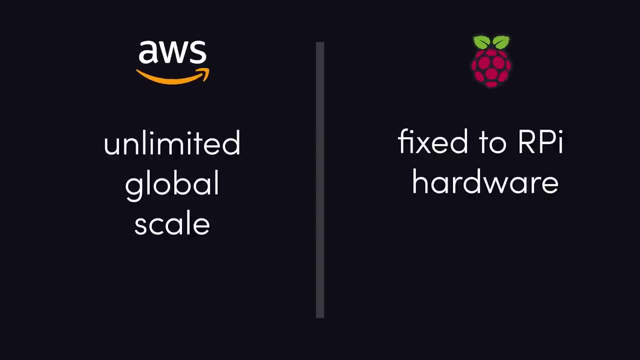 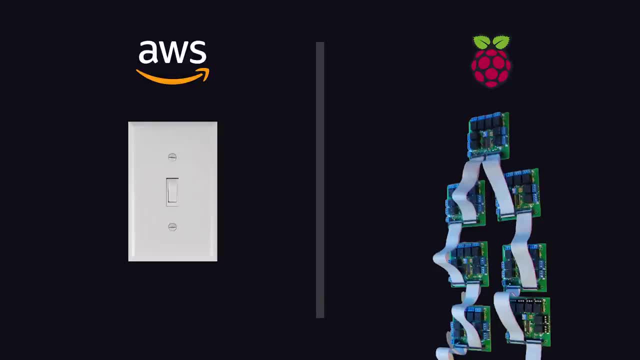 If we need to grow or scale up, we need to buy more Raspberry Pis and figure out how to distribute the load across them, And we'd likely want to do that in different parts of the world to make our infrastructure closer to the end user and also to provide fault tolerance, just in case some kind of 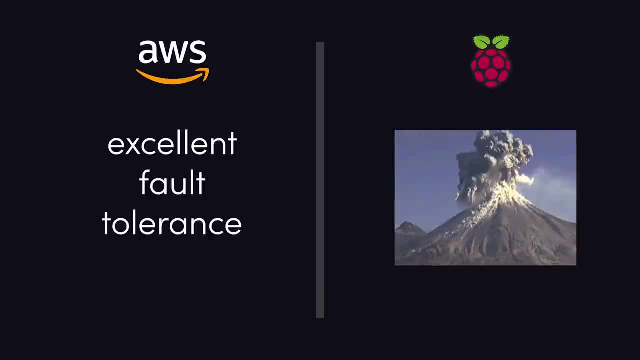 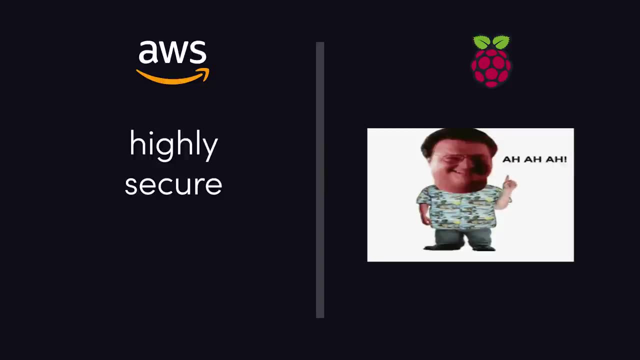 natural disaster destroys a Raspberry Pi like a volcano or peaceful protesters. In addition, we also need to think about security, Because we're dealing with a highly controversial app here. as soon as we go back online, every coder in the world is going to try to hack it to pieces. 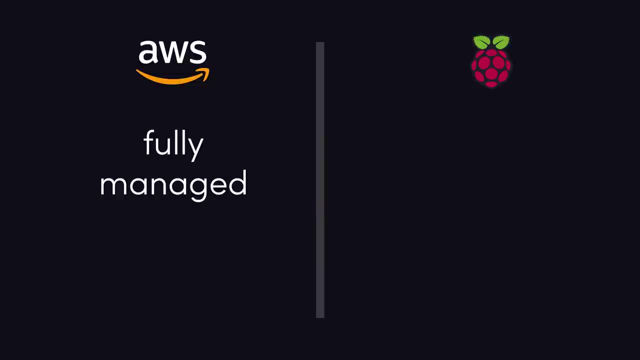 to save humanity from the buffalo guy. Another major drawback of this on-prem approach is that it takes a lot of manual configuration, Like we need to plug in cables, work with power companies to supply electricity, internet service providers to provide IP addresses, and the list goes on. 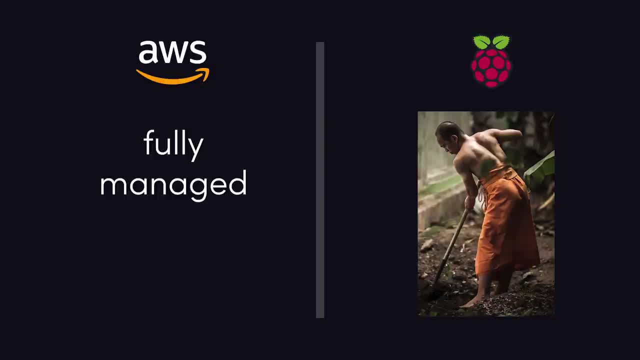 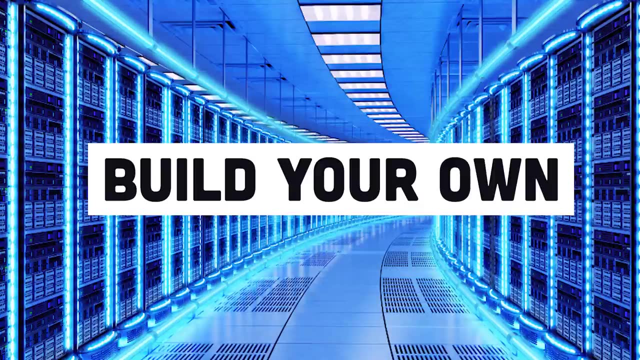 On the other hand, with AWS, we can do everything from a computer screen. it's all fully managed and much easier to work with. But once you're kicked off, you really only have two options: build your own data centers or file an antitrust lawsuit, Both of which are terrible options. 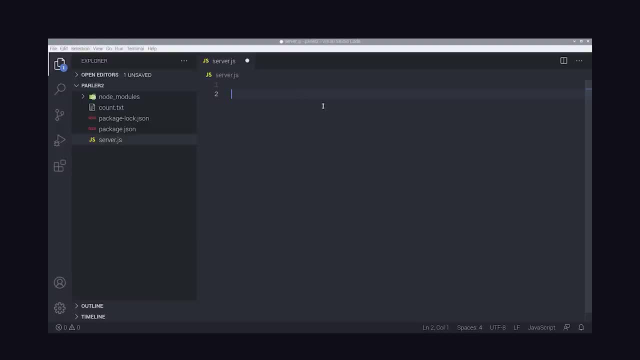 but let's go with the first one. From here. we're going to build a Nodejs app directly in the Raspberry Pi. It's a classic web page that tells you how many times the page has been viewed. Node is already installed, so we can open up an empty directory. 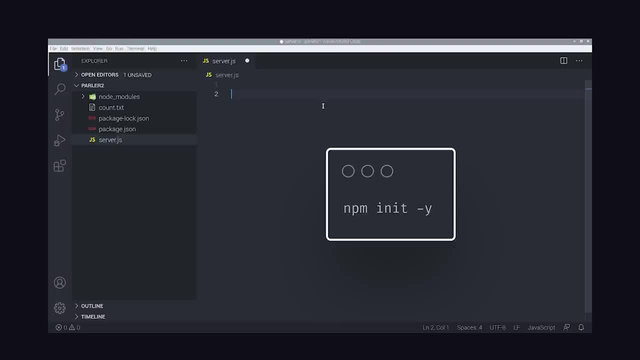 then run npm init y to create a new npm project. From there we can install Expressjs to help us build a web app. I'm creating a JavaScript file called serverjs for our main source code. Then, instead of a database, I'm just adding a text file to the project. 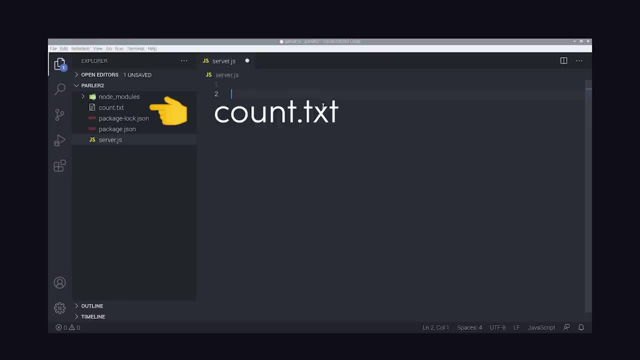 which we can read and write to to get the current count of people who have viewed the web page. In the JavaScript file we'll import ReadFileSync and WriteFileSync from Nodejs, then create a new Express app. The Express app will listen on localhost 5000. 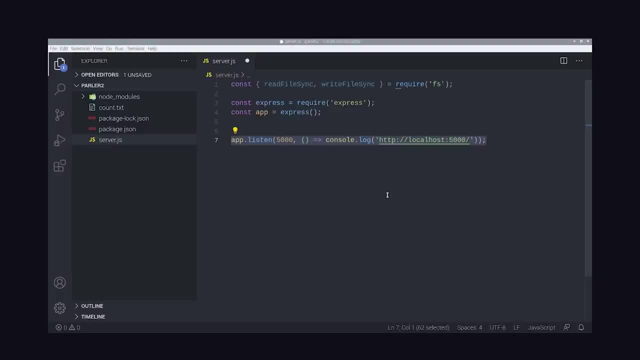 From there we just need an endpoint to the root URL. that will update the view count, then send back the raw HTML to the browser. In Express, we can create an HTTP endpoint by calling app get, followed by the URL, which, in this case, will just be the root URL. 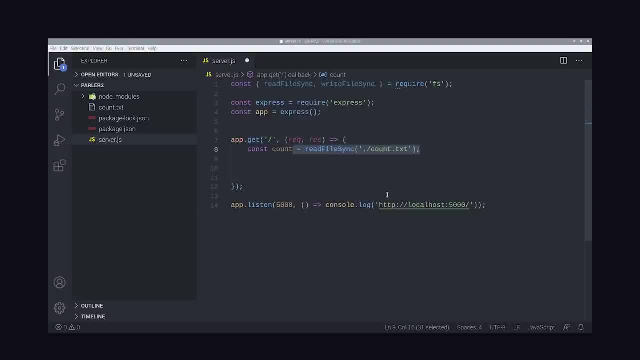 We can get the current view count by calling ReadFileSync, which will set to a variable Coming from a text file. it's a string, so we'll parse it into an integer, then add one to it. Then we'll simply write that value back to the same file. The final step is to send a response. 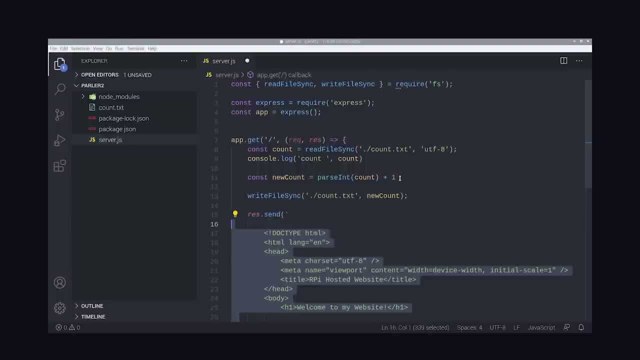 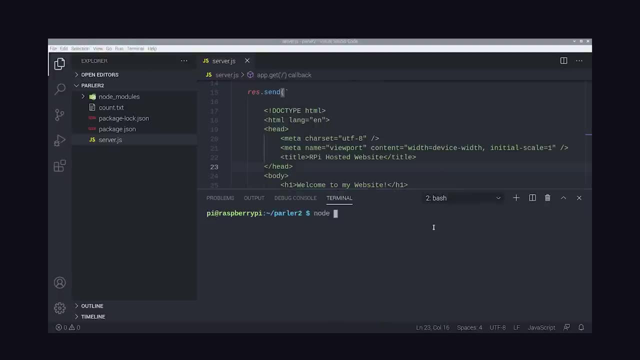 from the endpoint, which is just a raw HTML string, but we'll interpolate the view count into it so the user can see that in the UI. That's all it takes to build a web app. Now we can run it by calling node serverjs from the command line. Now, at this point, 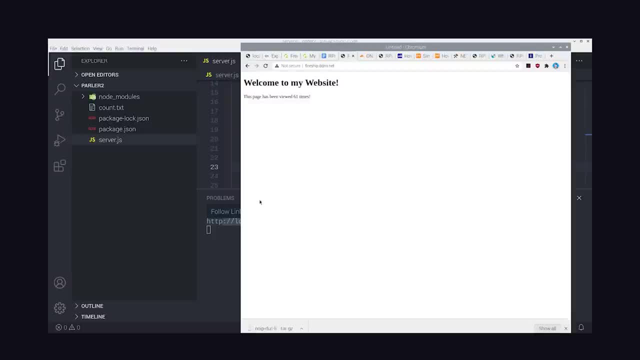 you should be able to open localhost 5000 on the Raspberry Pi browser and see your web app displayed here. At this point we have a working web app, but we're building a serious app here and that means we're going to deploy it with Nginx Once we add multiple Raspberry Pis to. 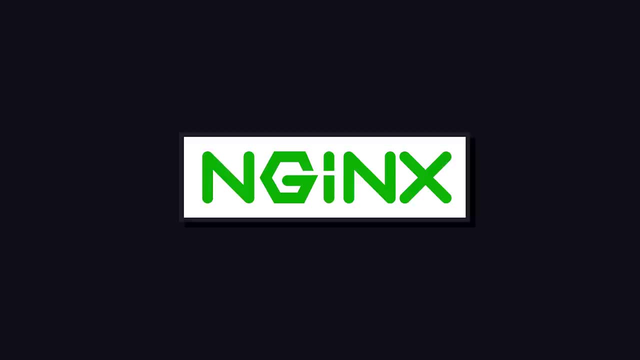 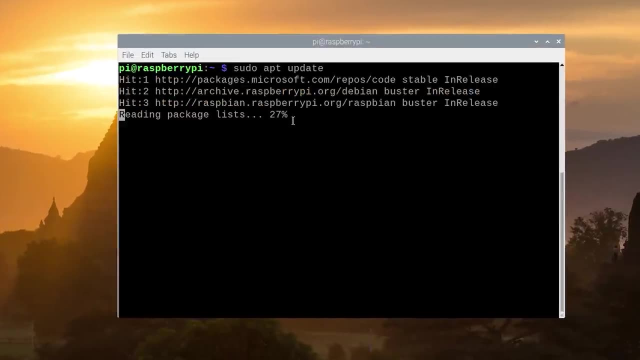 our data center, we'll be able to use Nginx to balance the load across them. Nginx is not installed on Raspberry Pi by default, so we need to open up the terminal and first run sudo apt update to get the latest information from the package manager. Then we can run sudo apt install. 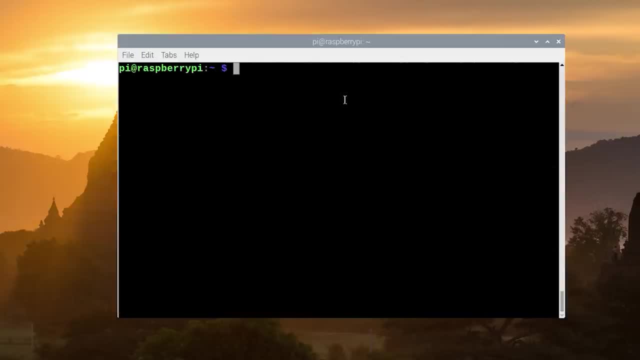 Nginx. This adds Nginx to the etc. directory, which we can run with sudo followed by the start command. This runs a default web page on the Raspberry Pi which we can access on its internal IP address. You can find the IP address by running hostname flag capital. I then paste that value into the. 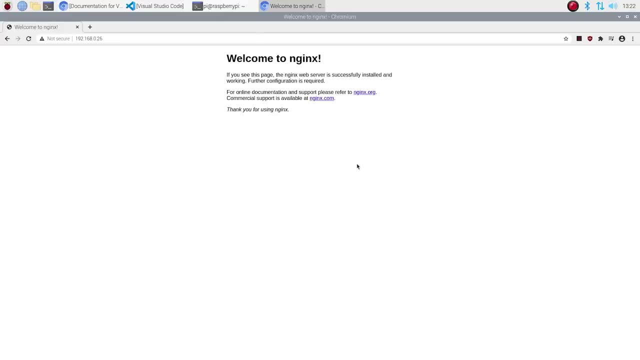 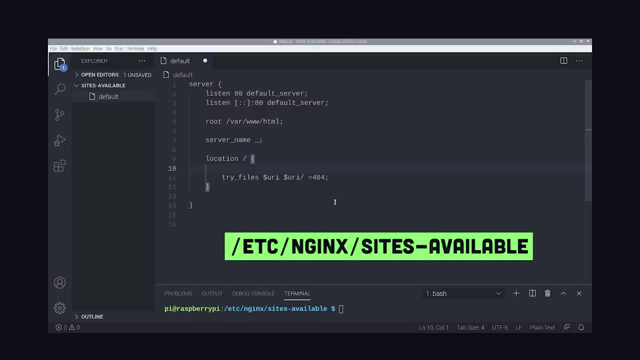 browser. It should say welcome to Nginx, but what we actually want to do here is proxy it to our nodejs application running on localhost 5000.. We can modify the default config in the etc Nginx sites available directory. I've removed all the comments, leaving only the default config. 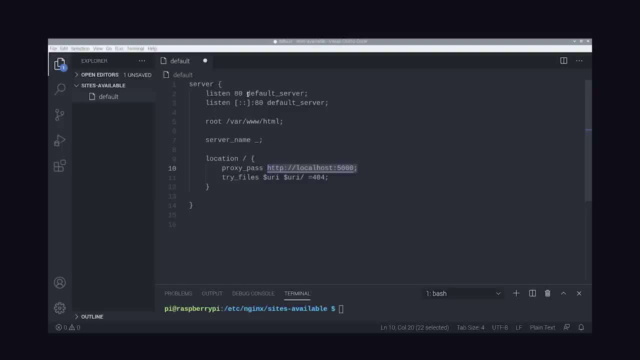 The only modification that we need to make here is to add the default config proxy pass to localhost 5000.. And that basically tells any traffic going to the root URL to use the nodejs app. save the file, then apply the changes by running sudo Nginx restart. Now that we have our 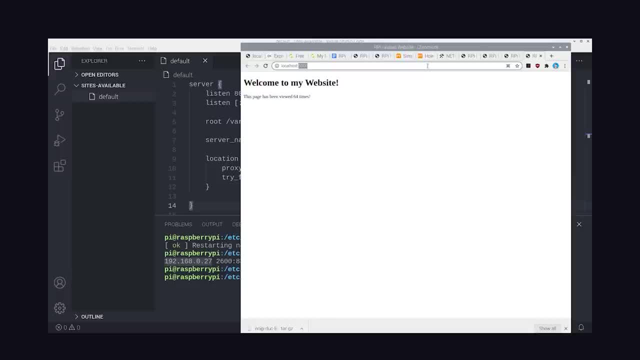 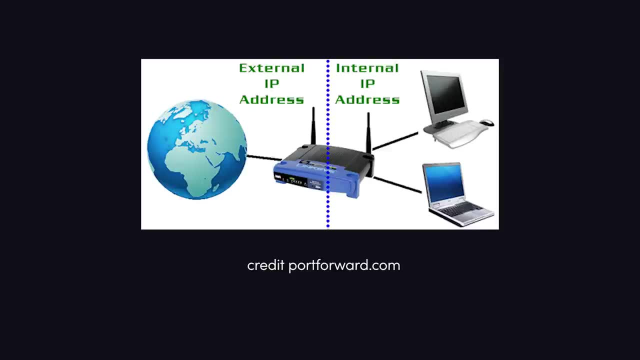 app running the way we want it on the Raspberry Pi, we need to make it available to the internet. The internal IP address can be used on your own local network, But in order to make the website available to the outside world on the internet, we need an external IP address, An. 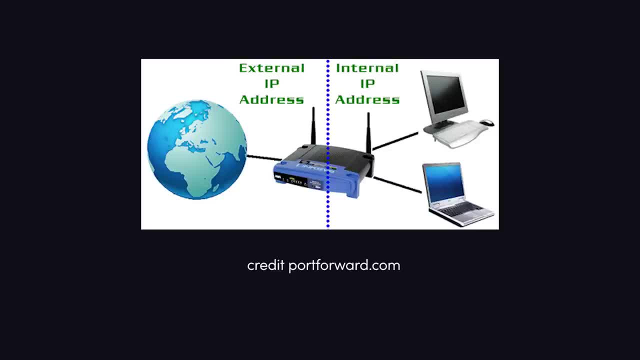 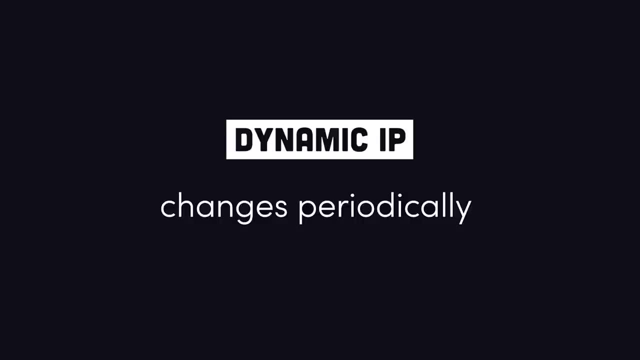 external IP address is provided by your internet service provider, like Comcast, Verizon, AT&T or whatever. For most people, they provide a dynamic IP address that can change on a regular basis. But it's not a great thing if you're trying to host a website, because once the 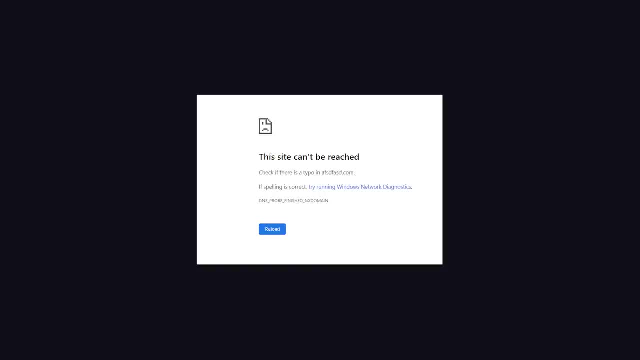 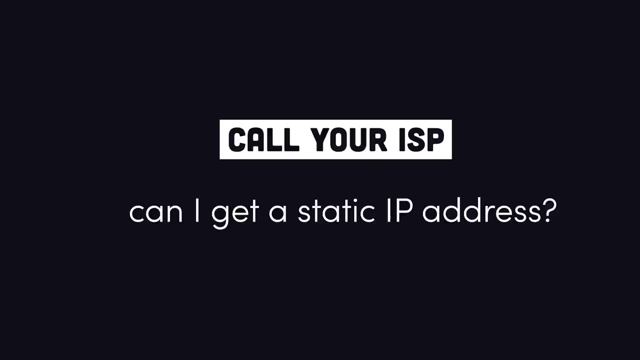 IP changes, then that means your website is no longer available on the internet. That means if we want to serve our web app from a Raspberry Pi, we have two options. We could call up the ISP and ask them for a static IP address. These guys don't exactly have a great reputation for. 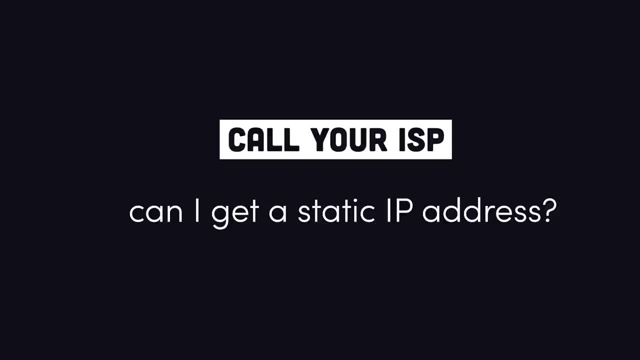 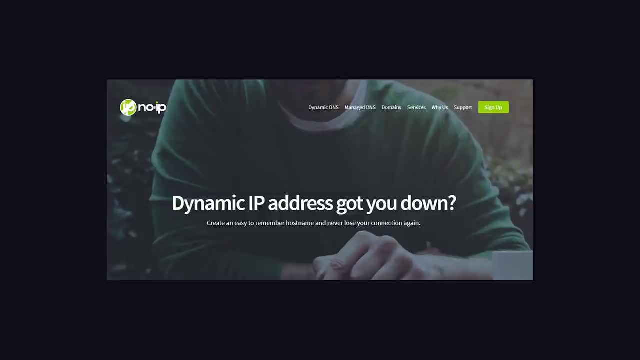 customer service, but getting a static IP from the provider is probably the best option. There are a few services out there that can monitor your dynamic IP and update it on the DNS for a domain when it changes. In other words, it makes your dynamic IP behave like a static IP. 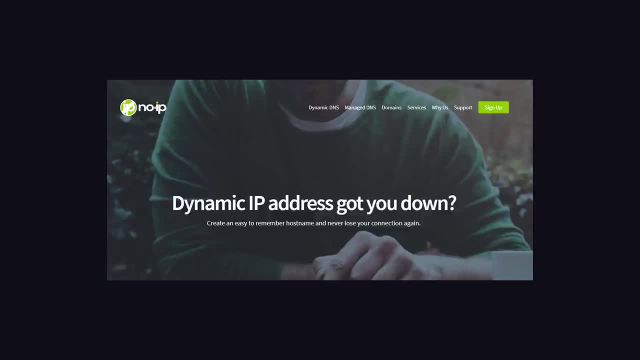 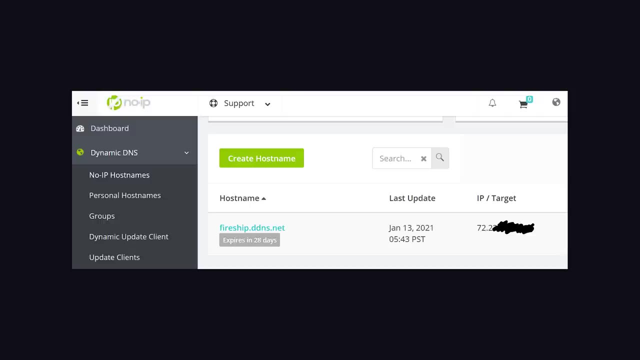 I'm going to be using noipcom because it has a free tier and it worked for me just fine. When you sign up, you pick a free domain name and it will automatically detect your external IP as the A record in the DNS. But in order for it to detect changes on the Raspberry Pi, 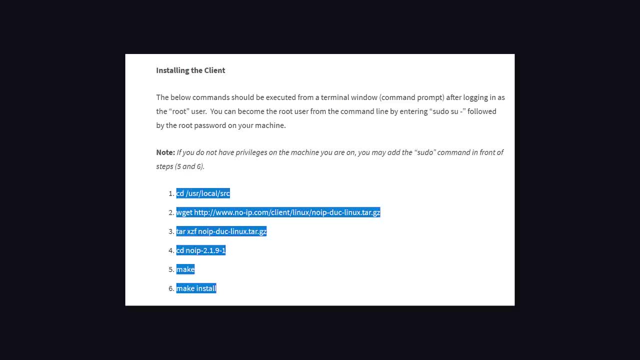 we need to install some software there. Basically, you just download a binary, execute it and then it will have you log in with your username and password to link the account to the Raspberry Pi. Once that's done, we effectively have a static IP, but there's still one more step left to get this thing working. If we try to. 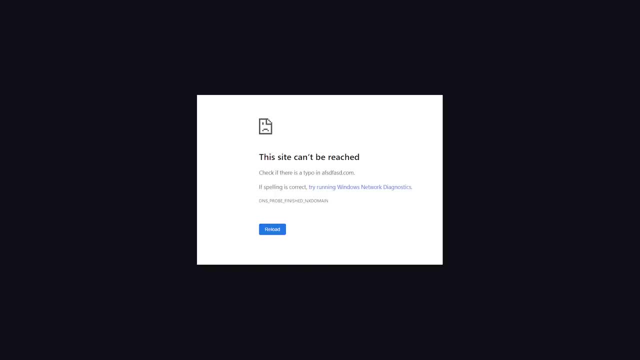 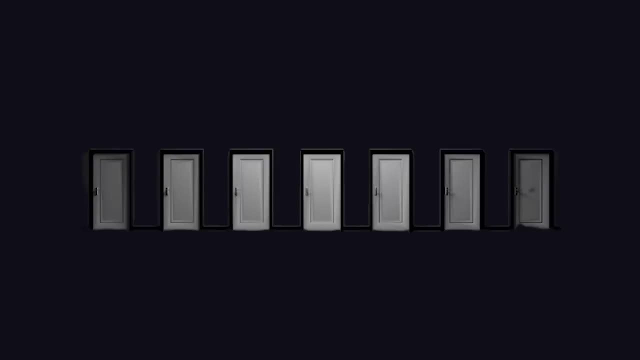 navigate to the external IP. at this point we get a blank screen. By default, your router will not allow outside traffic to get into your network. It's like a giant fence with a bunch of doors in it that are all currently closed. These doors are called ports, and our app is currently being served. 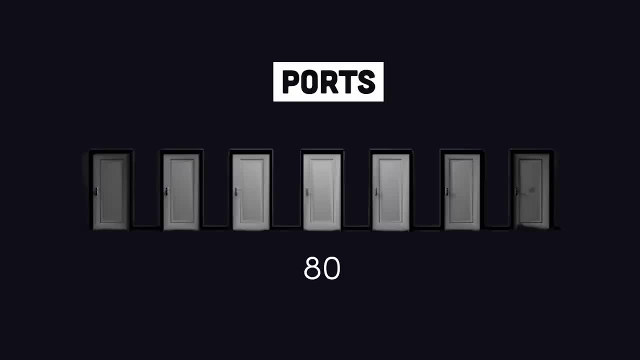 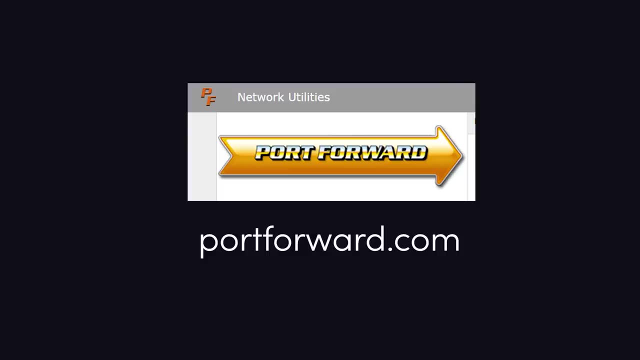 80. That means we need to open up port 80 on our router to external traffic through a process called port forwarding. The exact steps will depend entirely on the router you use, but there is a website called portforwardcom that has a breakdown for basically every router out there. 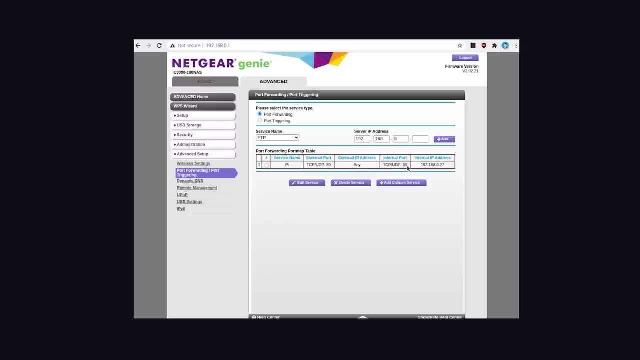 Once you connect to the router, you should be able to find port forwarding under the advanced options. What you'll do is add a new forwarding rule with starting and ending ports for 80 that connect your internal IP address to any external IP address. Remember, you can get your internal IP address by running hostname flag capital I from the command. 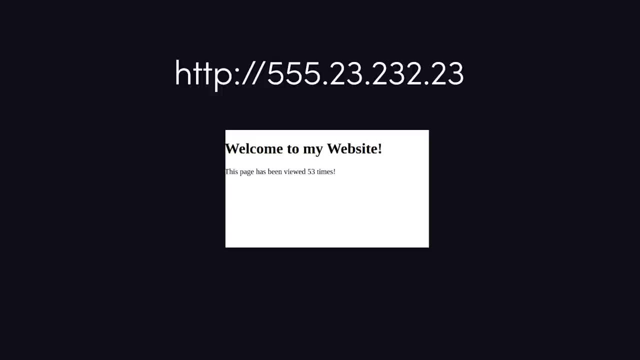 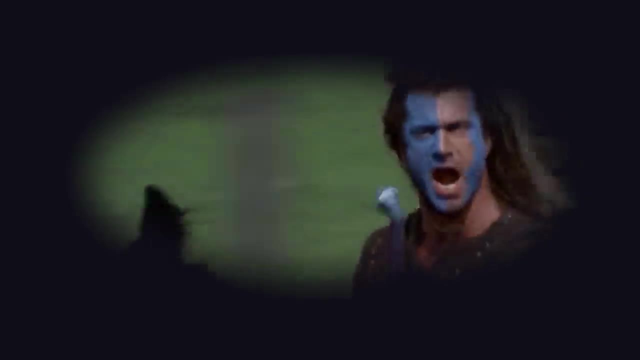 line. Once you have that done, you should now be able to navigate to your external IP address, and the result should be the Nodejs app that we built earlier. Congratulations: you just built your own Amazon Web Services from scratch. They may take our lives, but they'll never take our freedom.